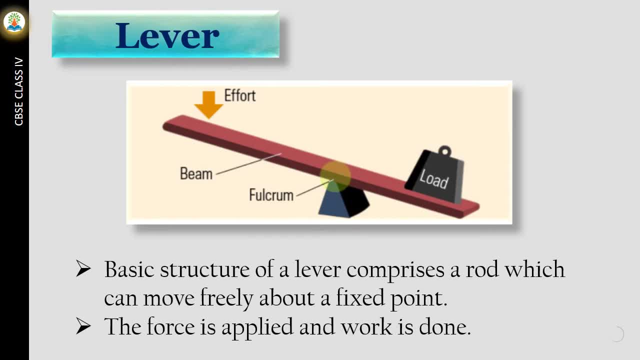 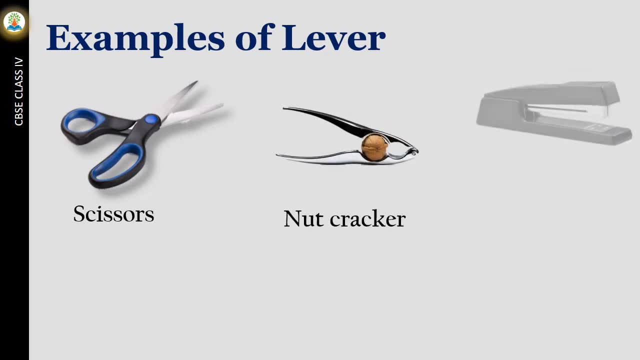 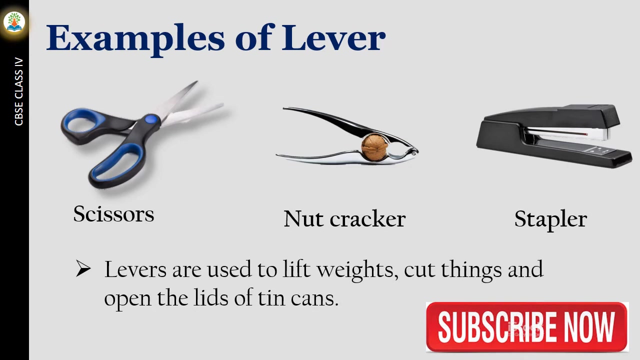 The force is applied and work is done. Machines are used to lift weights, cut things and open the lids of tin cans. The examples of lever are hammer, scissors, stapler, nutcracker and see-saw. Two wheels are attached to a rigid rod called axle. 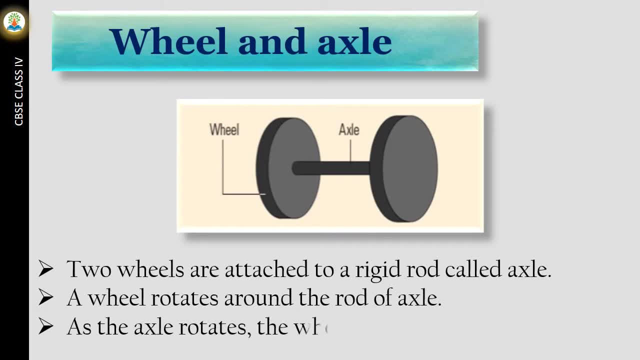 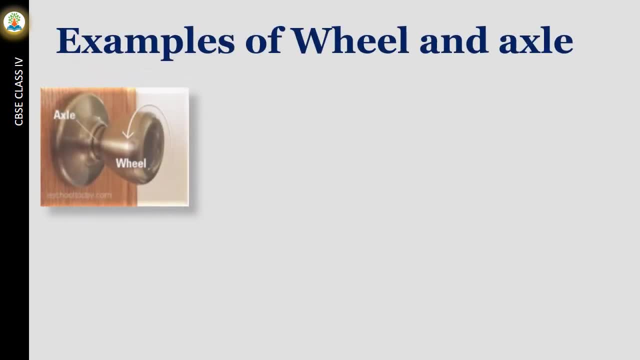 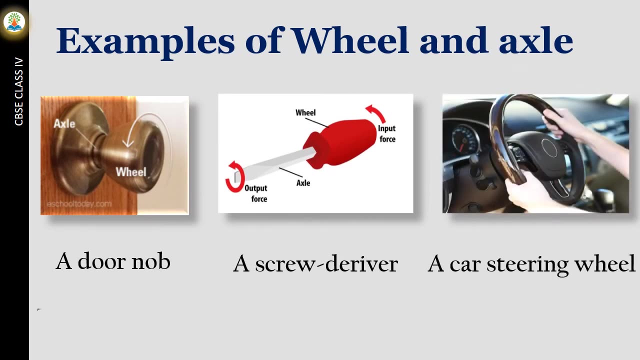 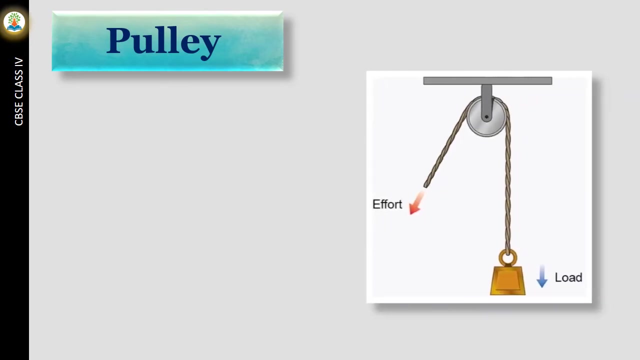 A wheel rotates around the rod or axle. As the axle rotates, the wheels also rotate. The movement of axle makes moving of heavier objects easier. A car steering wheel, a door knob and a screwdriver are the examples of wheel and axle. A pulley has a grooved wheel and a rope running between the groove of the wheel. 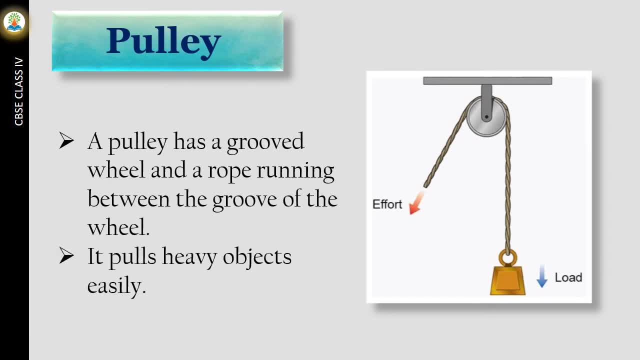 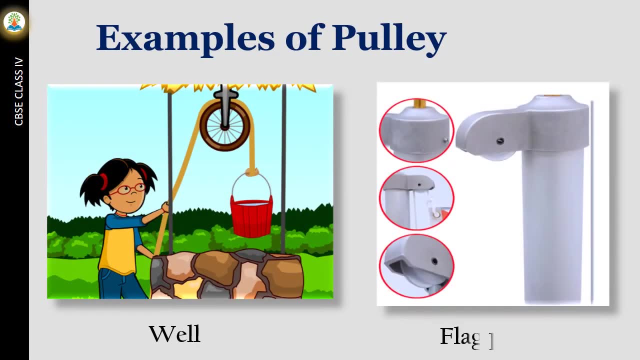 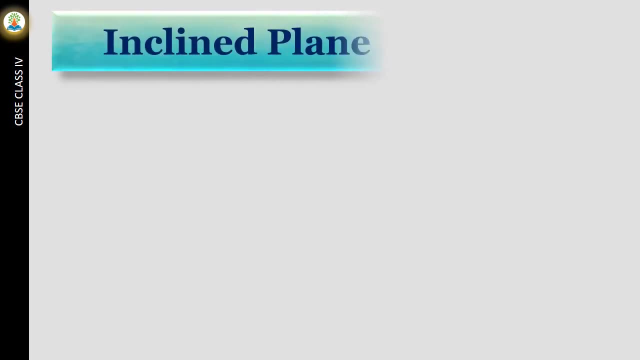 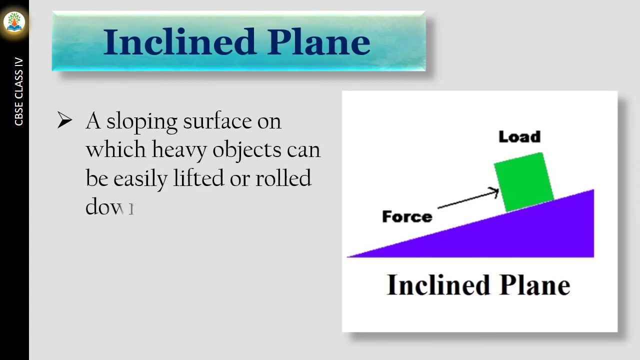 It pulls heavy objects easily. Examples of pulley are seen over the wells and at flag poles. A sloping surface on which the wheels are placed can be seen. A sloping surface on which heavy objects can be easily lifted or rolled down is called an inclined plane. 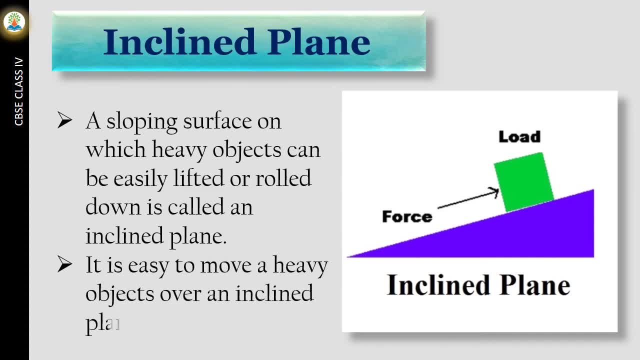 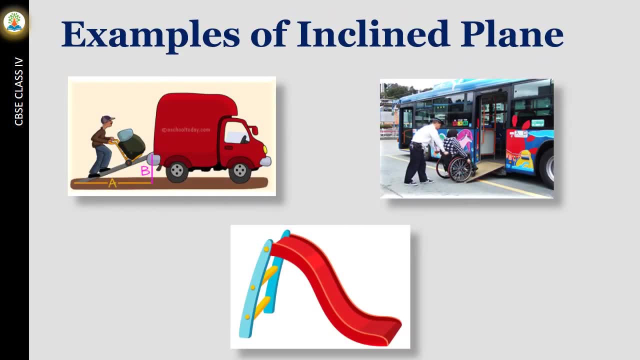 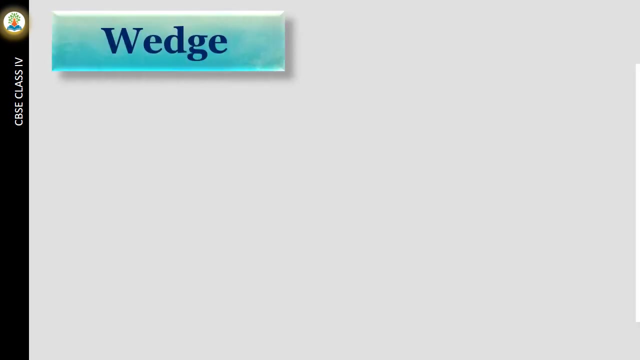 It is easy to move a heavy objects over an inclined plane. The patient are carried to the hospitals on stretchers or wheelchairs using a ramp, which is an inclined plane. Heavy cartons are loaded into trucks using inclined planes. When two inclined planes meet at a sharp and pointed end, a wedge is formed. 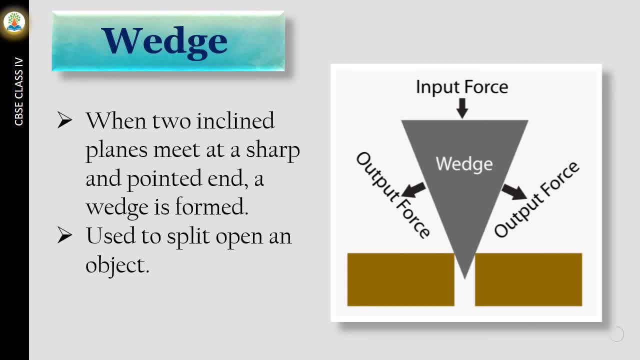 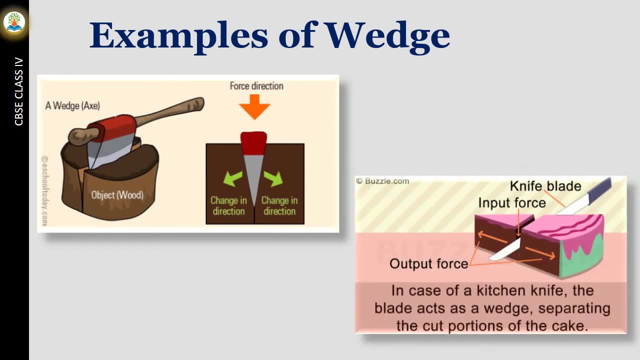 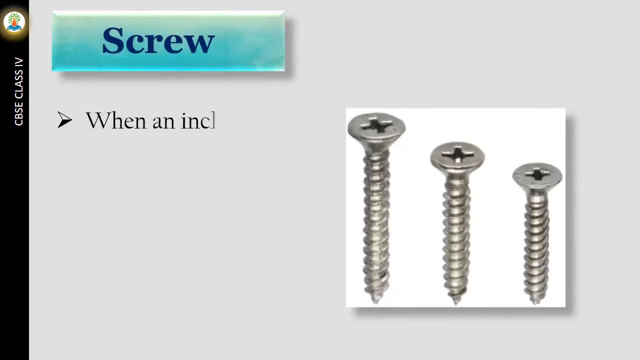 It is used to split open an object. The head of an axe and the cutting edge of knife are the examples of wedges. When an inclined plane is coiled around a cylinder that has a sharp pointed end, it forms a screw. It fits between objects and holds them together.